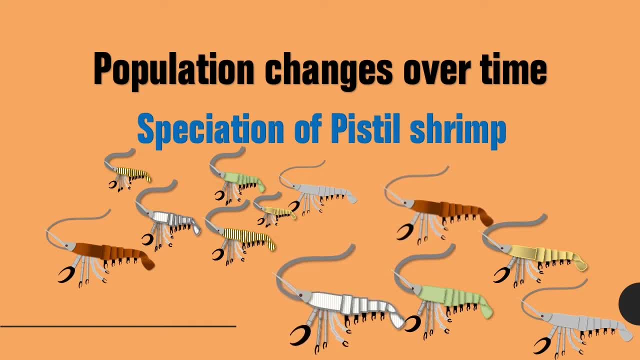 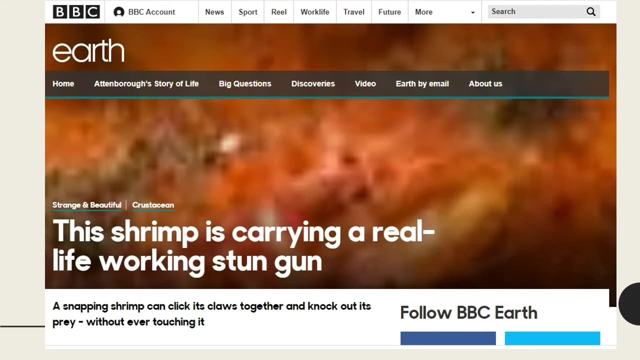 This claw can be closed at lightning speed. It will produce a loud snap as a way to either stun its prey, deter predators or communicate with others. The popping of the bubbles causes water to cavitate and even produce light, due to the high temperatures and pressure inside the bubble. 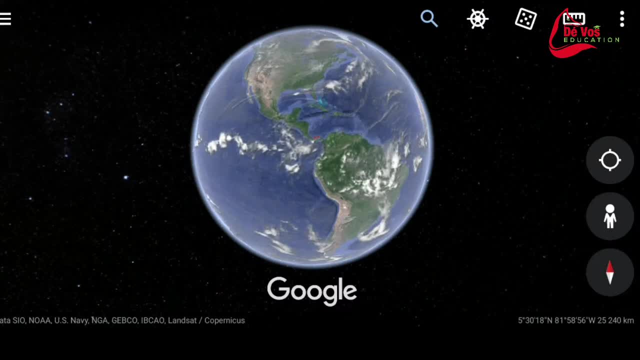 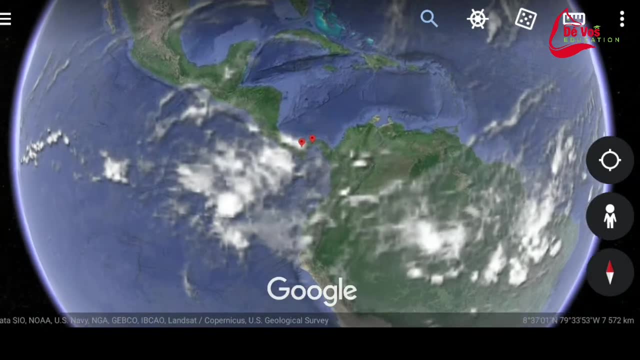 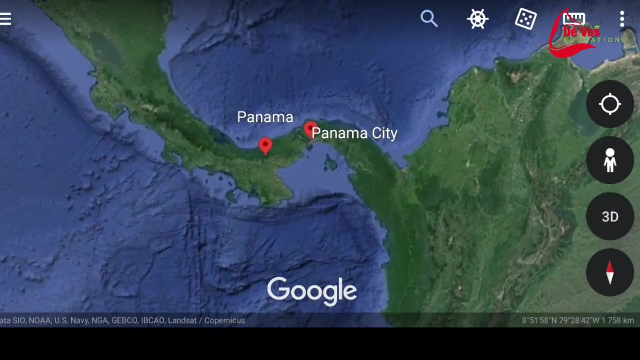 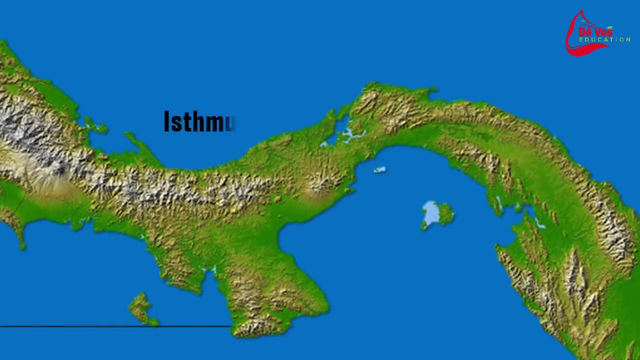 The sound they make is like the grilling of bacon or the crackling of burning twigs. We're going to look at the specific snapping shrimps found in the Panama Canal area. Long ago, the ocean flowed freely between North and South America. 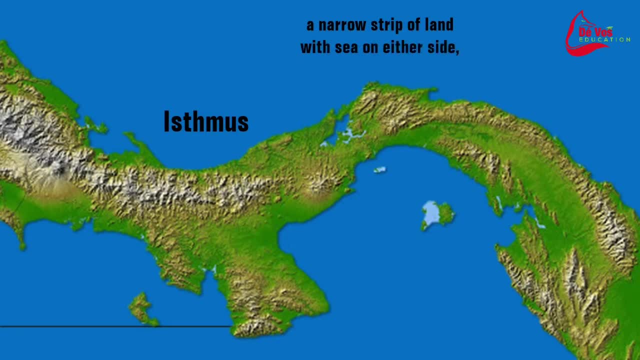 Then, approximately 2.8 to 3 million years ago, the Isthmus of Panama arose, creating a land bridge between the two continents. This is a narrow strip of land with a sea on either side, forming a link between the two larger land areas. 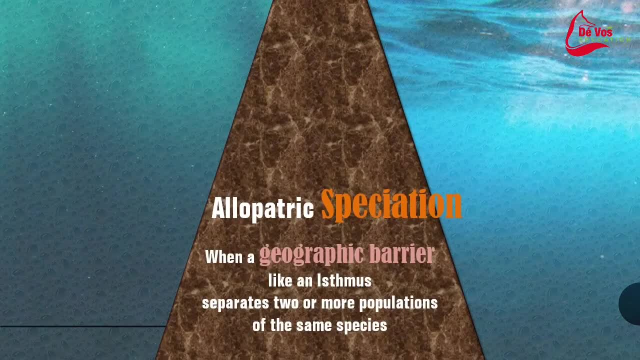 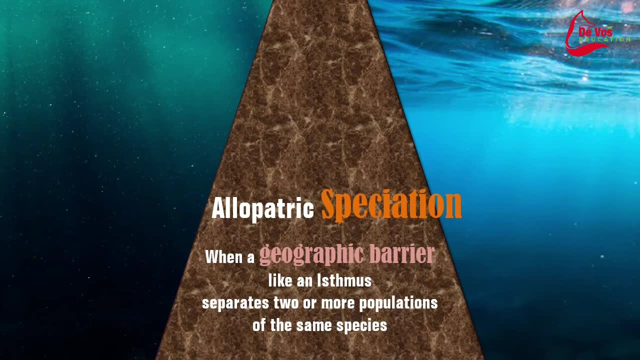 This is the Isthmus of Panama. This is the Isthmus of Panama. This form of speciation is known as allopatric speciation, and it is when a geographic barrier, like the Isthmus, separates two or more places. 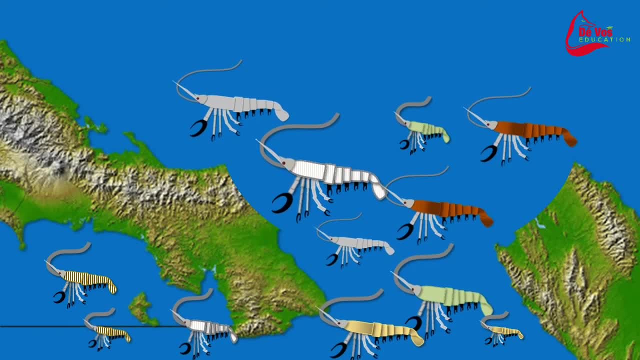 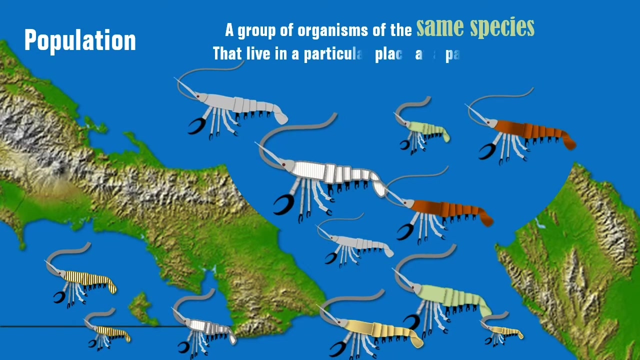 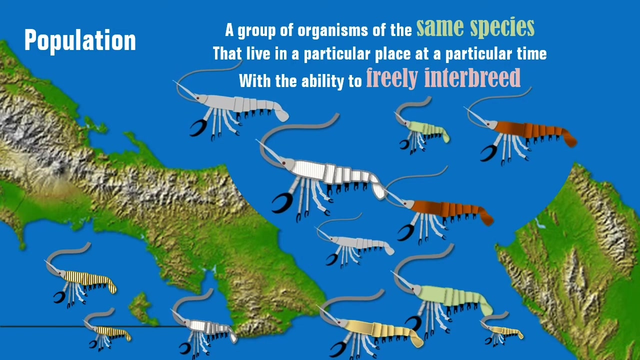 Originally, the populations of snapping shrimp were free to interbreed and move amongst themselves. The population is a group of organisms of the same species living in a particular place at a particular time, being able to freely interbreed. A biological species can be defined as a group of organisms that interbreed. 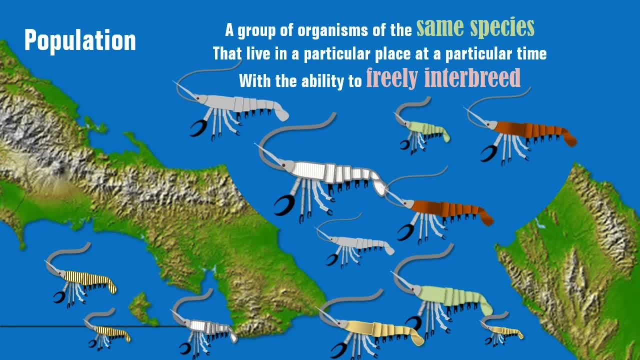 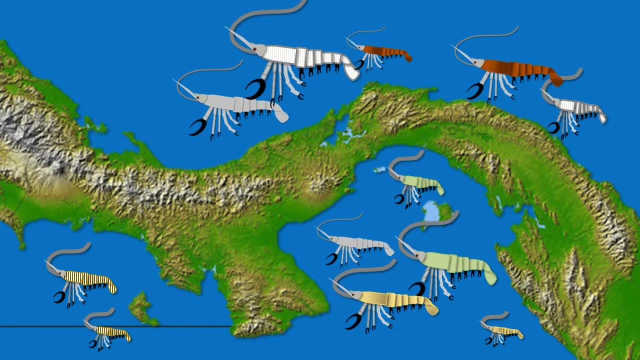 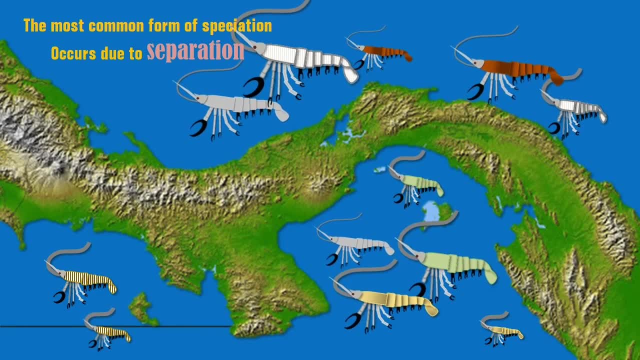 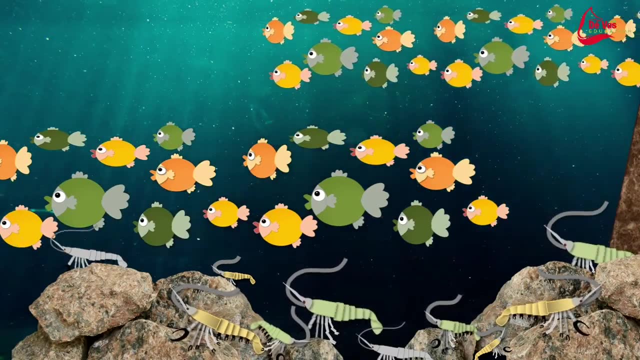 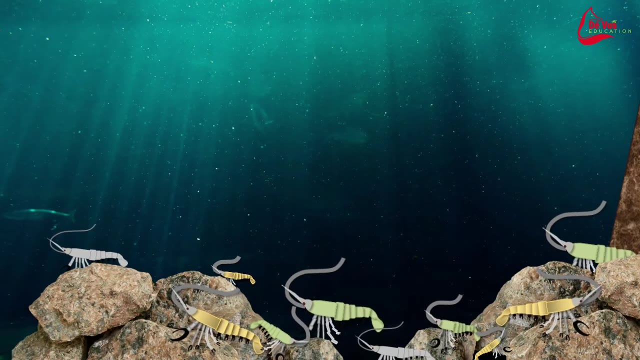 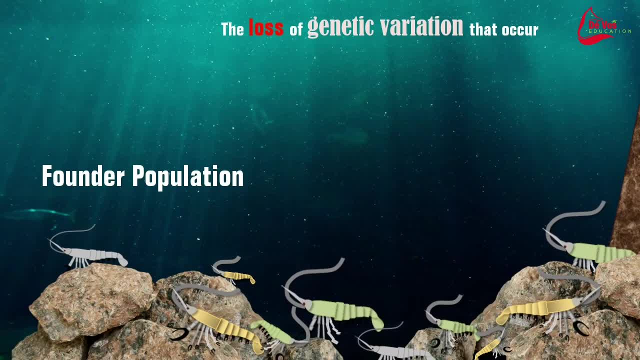 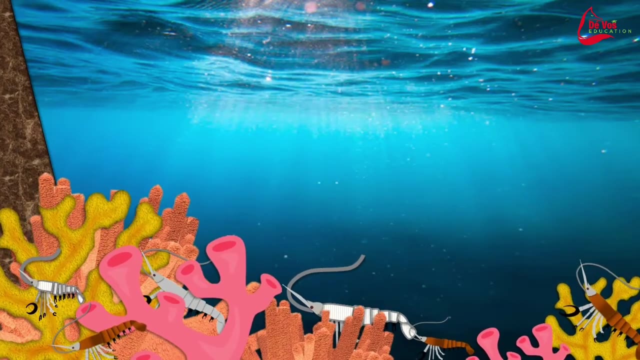 by this physical barrier. we talk about the founder population effect. There is a loss of genetic variation that occur when the new population is established with only a small number of individuals, with only a small number of individuals. Some others of these little organisms have mastered the art. 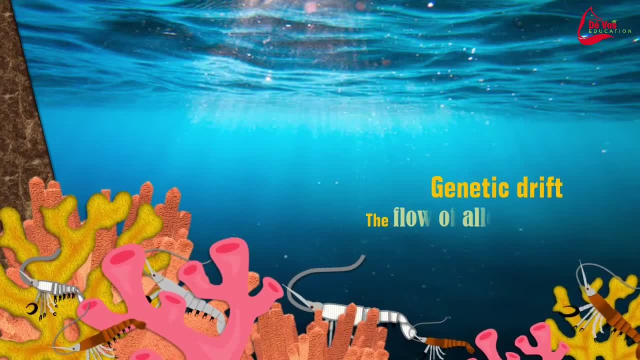 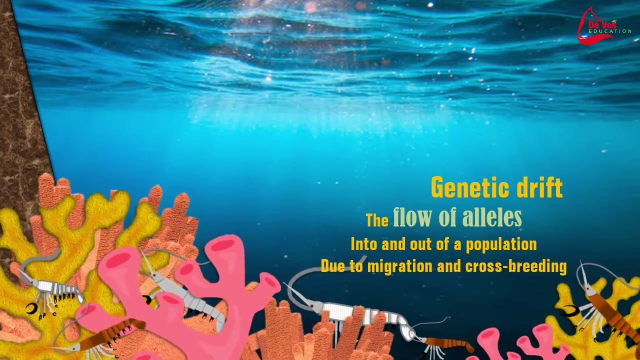 of symbiotic relationships teaming up with all kinds of little sea creatures. If there is enough genetic drift, there is a flow of alleles into and out of the population due to migration and crossbreeding. due to migration and crossbreeding. Due to migration and crossbreeding. 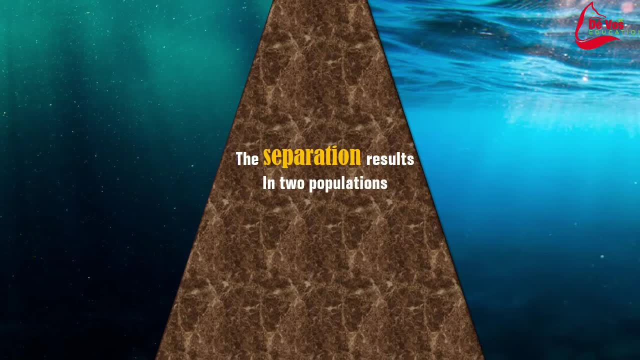 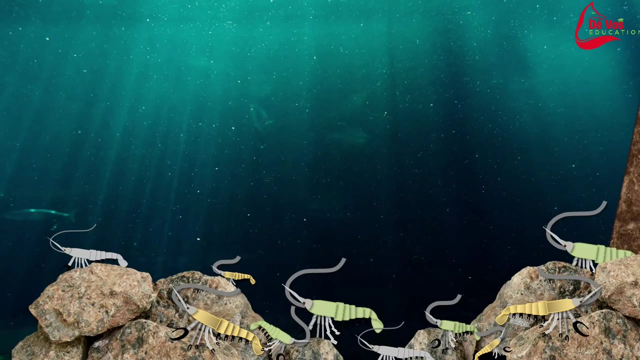 Due to the separation, it results in two populations that will be exposed to completely different environmental conditions. They develop in isolation from each other and they cannot crossbreed anymore. and they cannot crossbreed anymore In their different environments. they tend to live in colonies. 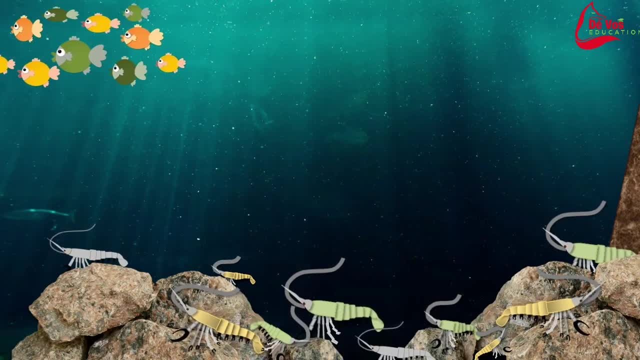 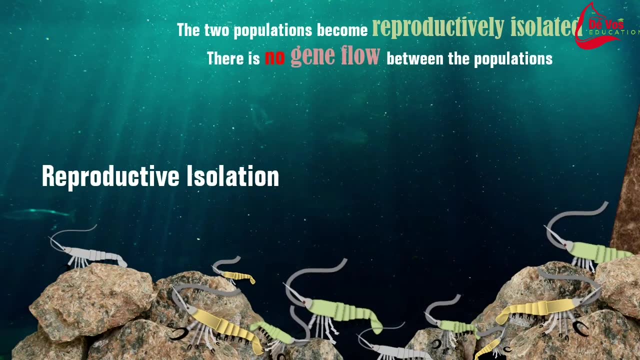 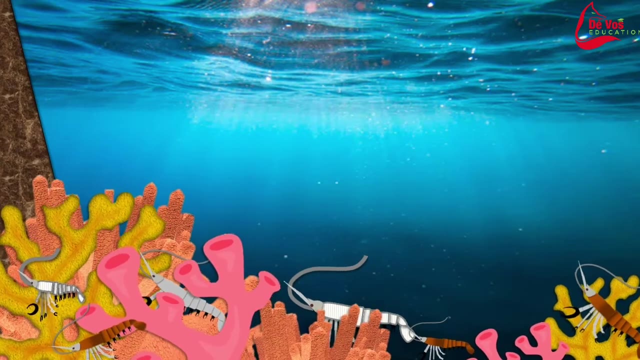 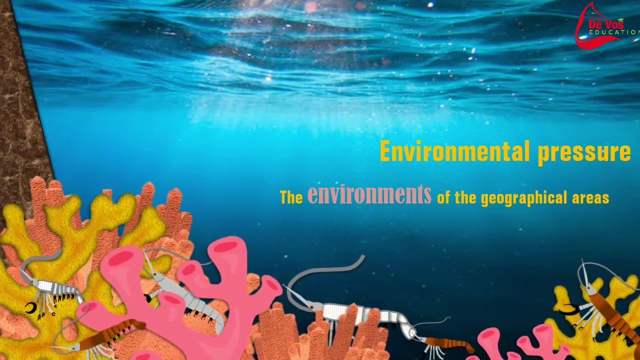 where they cluster close together. so if you listen, you can hear a whole chorus of snapping. This is then followed by reproductive isolation. The two populations become reproductively isolated from one another And there are the process of natural selection that also takes place.